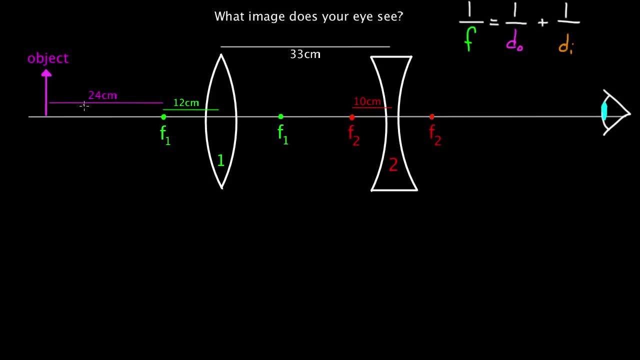 So we're going to add it over here looking through these two lenses. So let's do this First thing we've got to do. So I'm going to pretend like the second lens doesn't exist so it doesn't confuse me. 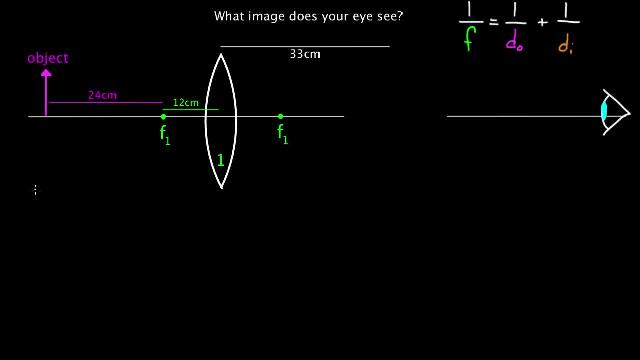 We use the thin lens equation. Alright, here we go. 1 over f, so 1 over. okay, here we go 12 centimeters. Do I make it positive or negative? It's on the left. Maybe I make it negative. Nope. 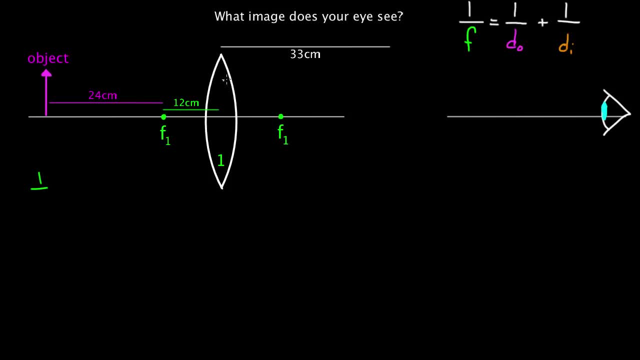 The only thing you look at is what kind of lens this is. This is a convex lens. You can tell by the way it's drawn. Since this is a convex lens, my focal length is going to be positive 12 centimeters, So that's what I plug in. 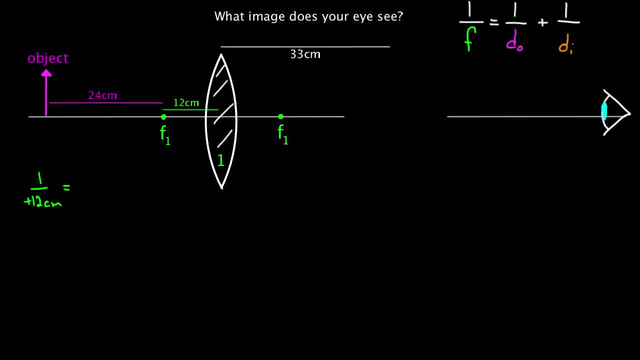 Positive 12 centimeters equals alright object distance. So 1 over the object distance, that's 24, right? No, All distances are measured from the center of the lens to the thing you're looking at, And so for an object distance I'd have to go from the center of the lens all the way to the object. 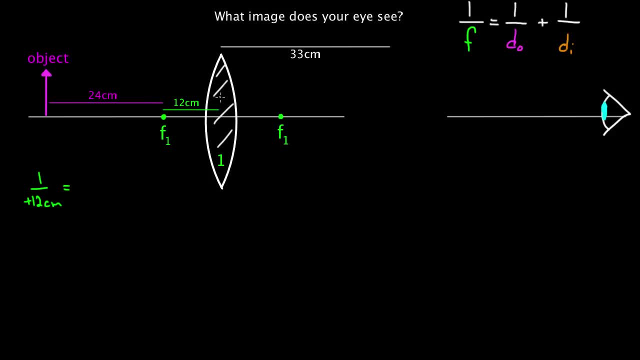 Don't just plug in any number they're giving. you Got to plug in that distance and that's going to be 24 plus 12. It's actually 36.. So I'd have 1 over and this is going to be 36 centimeters, positive or negative. 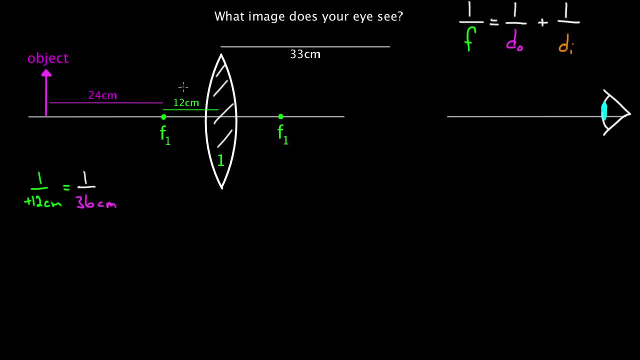 Well, that's going to be positive. here. We've got two lenses, but for this first case it's on the left-hand side, Everything's cool. It's on the opposite side of my eye. It's going to be a positive 36.. 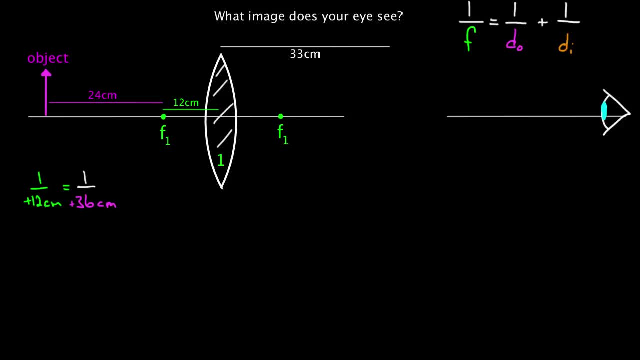 I'll show you in a minute how this could possibly be negative in a second. Plus 1 over the object distance, The image distance. I'll just label that with a DI. Alright, so now we've just got to solve. If you solve this, you're going to get 1 over 12 centimeters minus 1 over 36 centimeters equals 1 over DI. 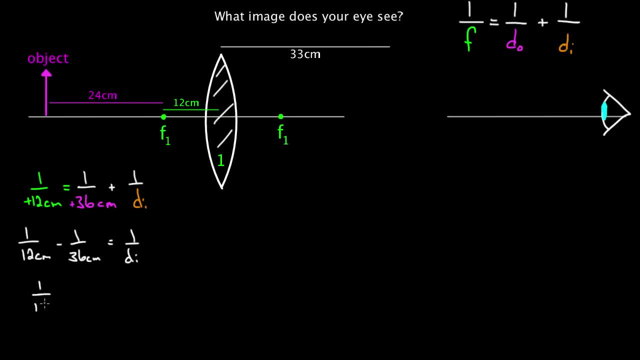 What you're going to end up getting is 1 over 18 centimeters on the left-hand side equals 1 over DI, But that's 1 over DI. If you solve that for DI, you'll get that DI equals 18 centimeters positive 18 centimeters. 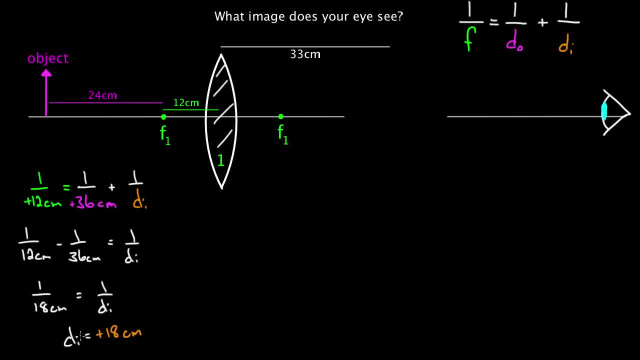 And so what does that mean? Where is this? Well, alright, DI. positive image distance. Remember, positive means on the same side as your eye for a lens. So I'm going to be, I'm going to have an image that's formed over on this side of the lens. 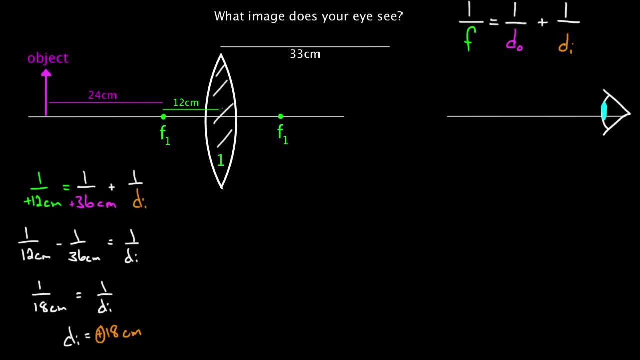 And 18 means 18 centimeters from where? From the center of the lens. So if I draw this, I'm going to go 18 from here. That's going to be past the focal point, Because I know the focal point is only 12.. 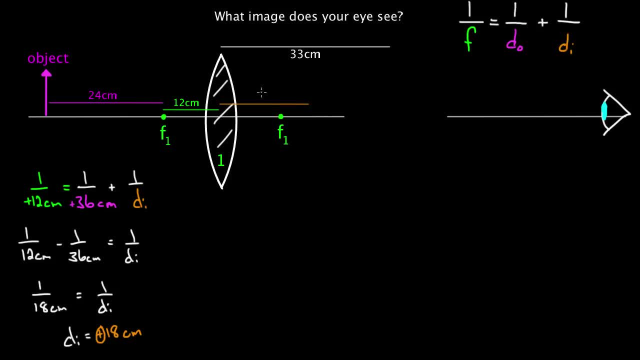 So I'm going to be somewhere around here, I'm going to label that That's going to be 18 centimeters And that's where the first image is. So that's where the image is going to be that this first lens creates. 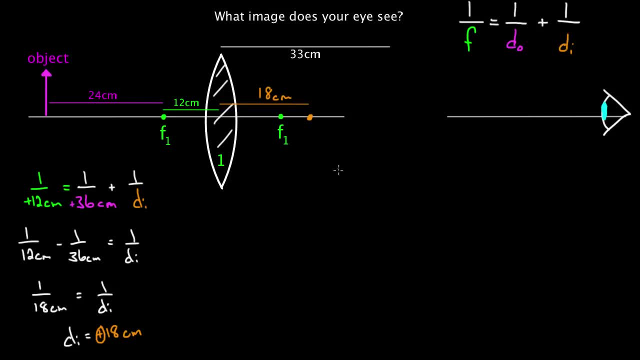 It's going to be right there, Okay, so now what do I do? I told you here's what we do: We pretend we'll bring the second lens back. We know the image that the first lens created is right here. 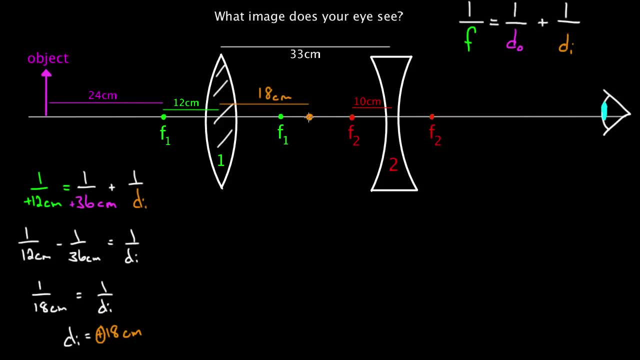 This second lens is going to think that that's the object. It's going to create an image of that image as if that were an object. So we do another thin lens formula, But this time we treat this positive 18, not as if it's the image. 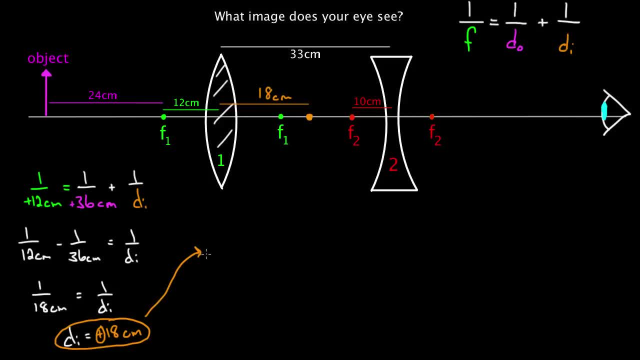 We treat it like it's the object. So this is going to be well, it's not going to be exactly equal to DO Because, remember, you have to measure everything from where? From the center of the lens. So for this second calculation, 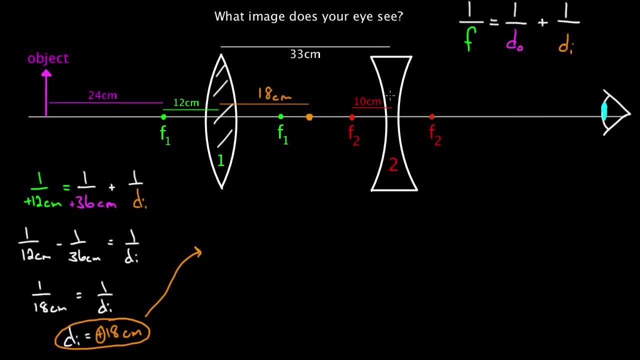 My object distance is going to be from the center of the lens all the way to- Let me not use that color. Let me see, Let's pick this one here- From the center of the lens all the way to where its object is. 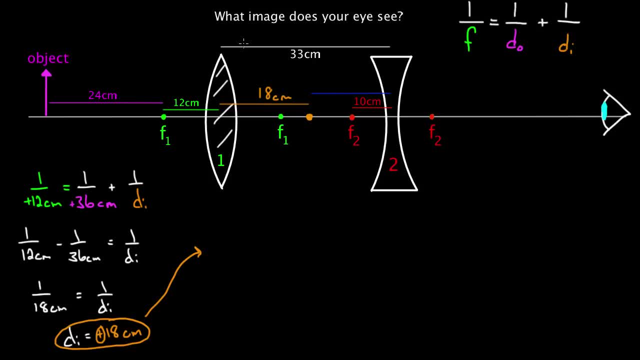 And its object is over here, which is not 18.. That's why I gave you this distance between lenses. The distance between lenses is 33 centimeters, So if the distance from this first lens Is 18.. Well, the difference has to be equal to this length. 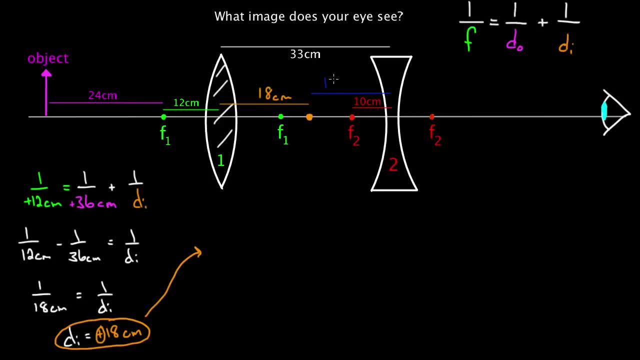 So 33 minus 18 is going to be 15.. Whoops, 15 centimeters will be where the object quote unquote for this second lens is going to be. So we turn this positive 18 into object: distance of positive 15 centimeters. 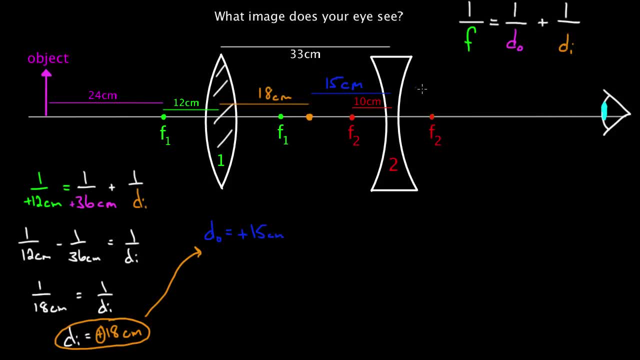 Why positive? Well, it's still on this left hand side. Opposite side is your eye. That's where the objects are supposed to be. Now, here, this is where I told you There's one case where you can get negative object distances. 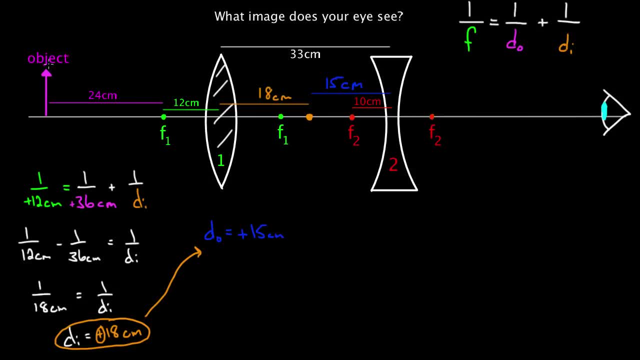 If our first lens would have created an image of this object way over here, On the wrong side of the lens, In other words, if this first lens created an image that was closer to our eye than the second lens was. Well, that's just all messed up. 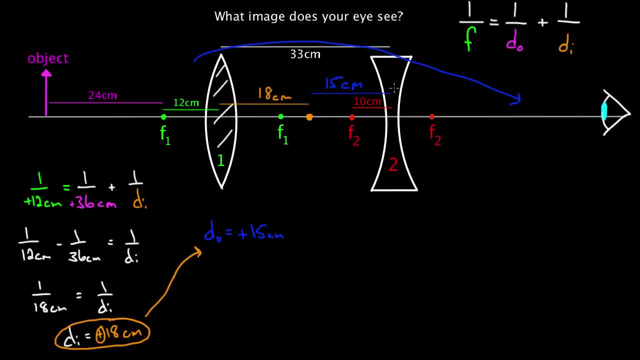 That's going to be a negative object distance, This object. You're not supposed to hold an object between your eye and the lens, So we'd count that You'd do your calculation just the same. I mean, everything would work out right. 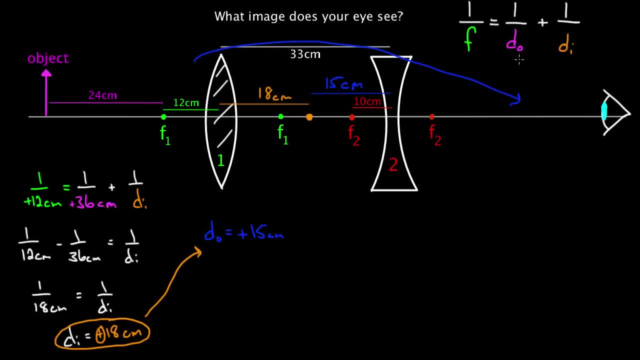 It's not like the whole thing is going to break. You'd get an image. It's just when you do your calculation. for this second case, If your image ended up on the wrong side of the lens For the first image, that was created. 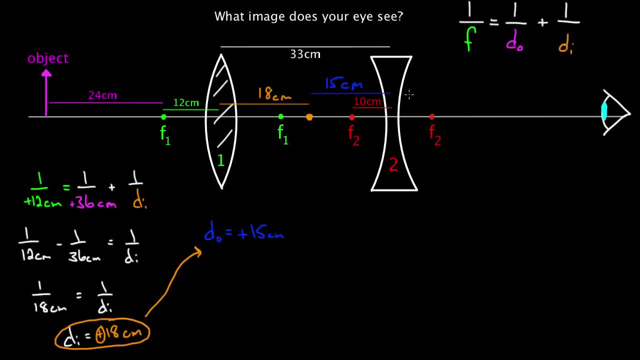 You'd have to treat it as a negative object distance. That didn't happen here. Our image is still formed on this side. We're going to pretend, See, We're going to pretend like this first lens didn't exist. We got an object over here. 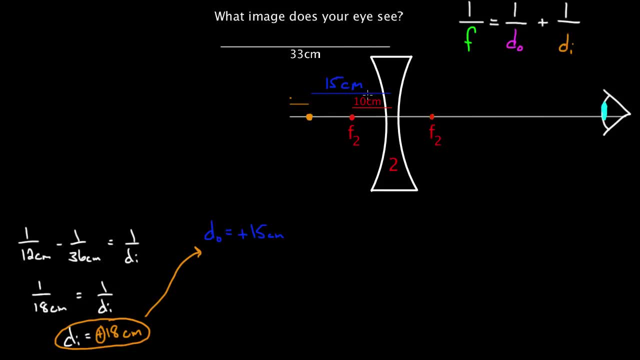 We're going to treat it like our object. Everything is fine Eye looking through the lens at our object. So we still treat this as a positive 15.. So let's do our calculation. We'll have for this lens It's going to be 1 over. 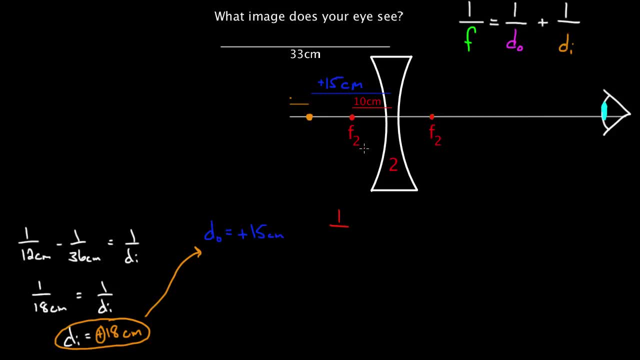 Alright, Focal length. What do we look at for focal length? We look at what type of lens this is. This lens is a diverging lens. Diverging lenses always get contributed, Always have a negative focal length That they contribute into this equation. 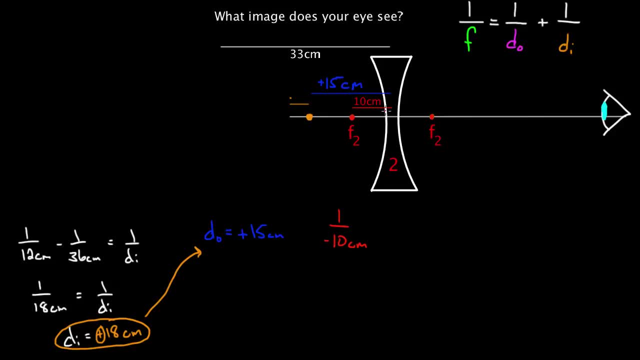 So a negative 10. Centimeters- That's the focal length of the second lens- Equals 1 over our object distance. we just found It's not really an object, That's okay. It's an image. But this lens doesn't know that. 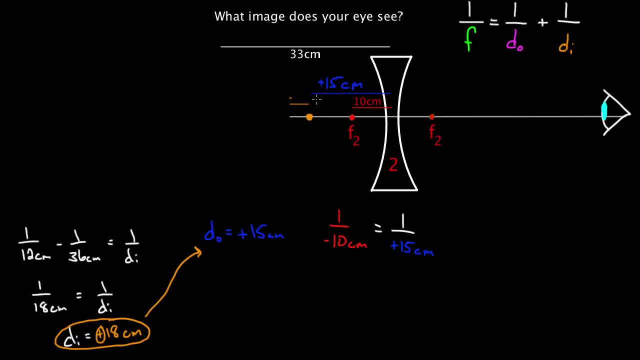 It thinks it's an object, So 1 over positive 15. Because it's still on the side that that object was supposed to be on, Plus 1 over our image. This is going to be a second image. This is the second image that this lens system has. 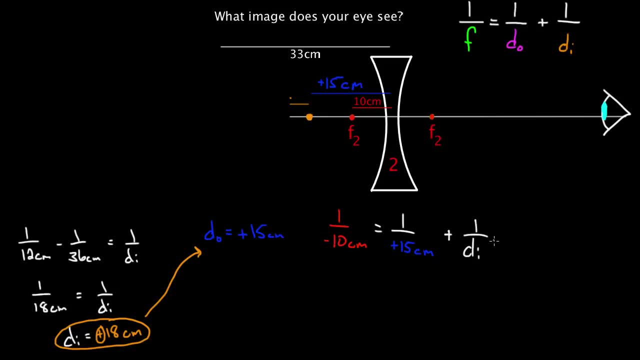 That this lens system is going to create, And so I'll just put DI: Alright. So we do the math Alright. 1 over negative, 10. Centimeters Minus 1 over 15. Centimeters Equals. 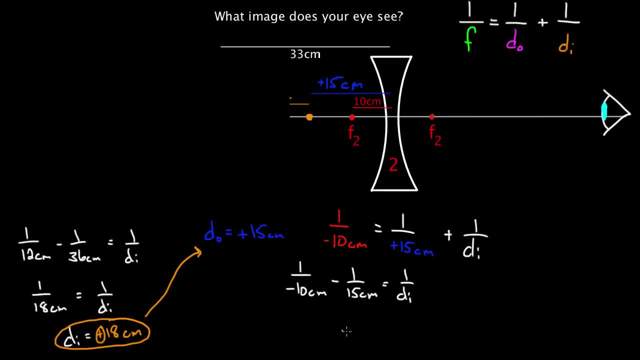 1 over DI. You solve that on the left hand side. You flip it over. You're going to end up getting that DI is, Once you do that inversion, Negative 6. Centimeters: That's what our second image is going to be. 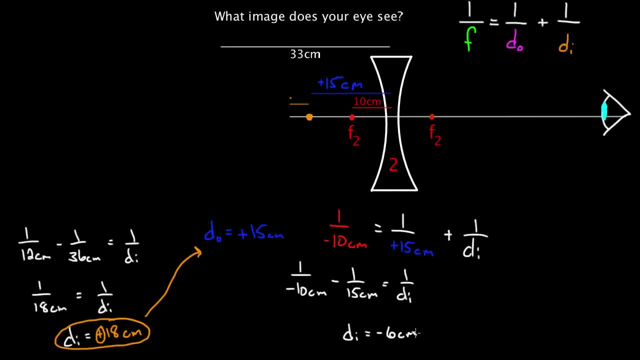 So what does this mean? Negative, 6. Centimeters, This is always from the lens, And negative- Remember negative image distance means on the left hand side Or the opposite side of your eye. So I'm going to come up here. 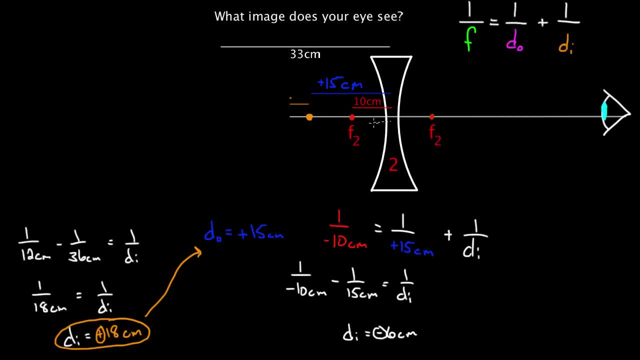 And I'm going to draw a line that goes from the center of my lens 6 centimeters to the left, Somewhere around there. That's going to be 6 centimeters right here. Whoops, I'll label that. That's going to be 6 centimeters. 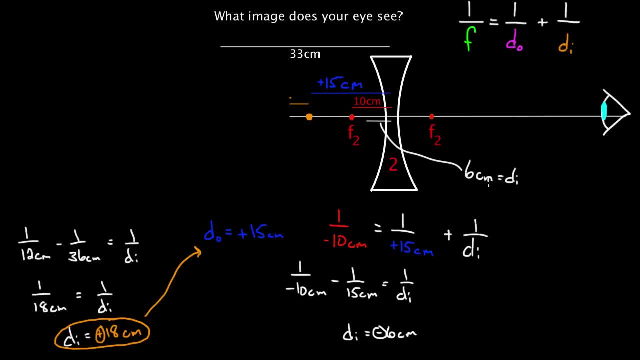 Because that's our image distance And that means our final image is right there. Our eye is going to see an image of something, Our arrow right at that spot, right there. That's where our image is going to be. And just to recap what happened: 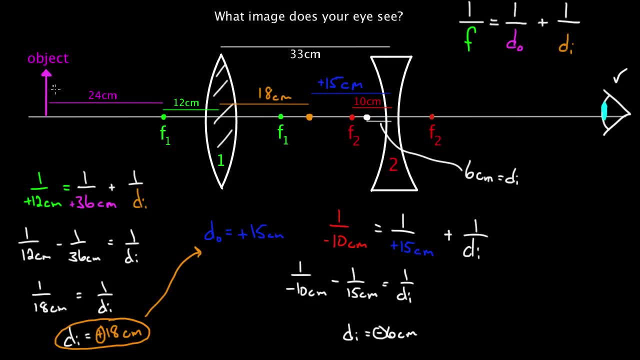 Whoops. So this first lens created an image of the object Over at this point here, This 15 centimeter point, And then the second lens created an image of that image. It treated it like it was an object And it created an image at this white point right here. 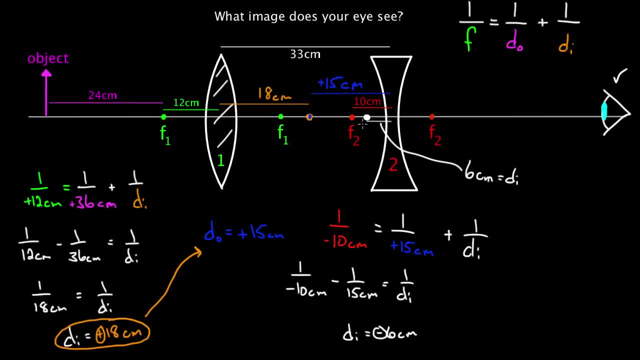 That's where we're going to see the image, But we don't know what it's going to look like. These calculations, This thin lens formula, only shows us where the image is going to be. If we wanted to figure out how big it was, 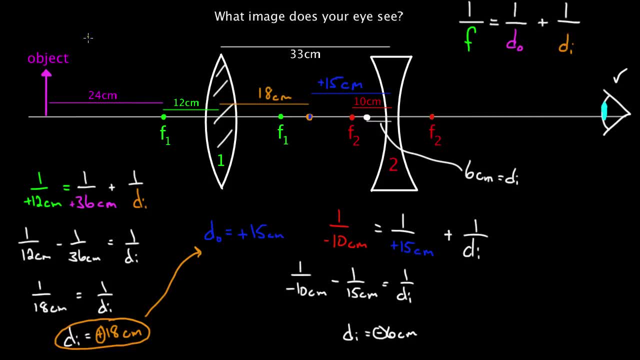 We have to use the magnification formula. So let's do that Over here. Magnification equals negative DI. Remember it's negative DI over DO. Alright, What was DI for this first case? We're going to do it one step at a time. 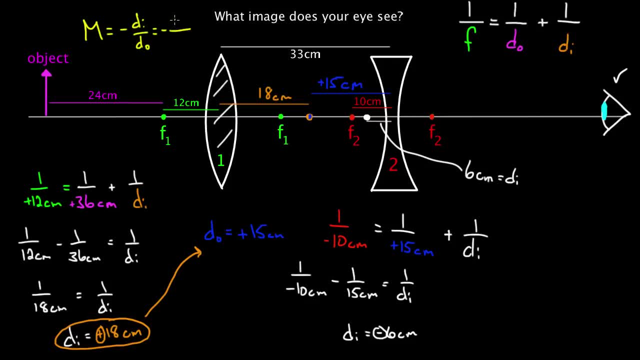 For this first case, The DI was positive 18.. So I'm going to put positive 18 up here. I'm going to leave off the units because they're going to cancel. DO was not 24.. It was 36.. So what do I get? 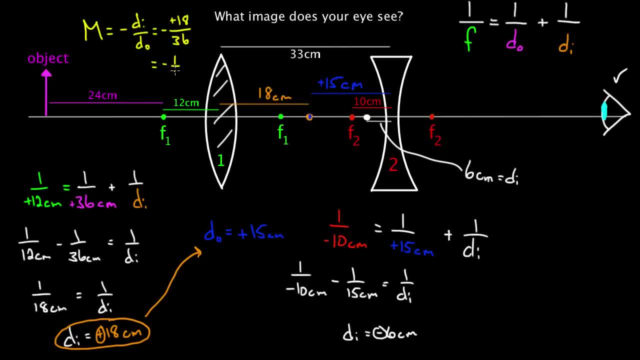 I get negative 18 over 36.. That's one half Negative one half. What does that mean? That means this first lens, The image it created is going to be An image that's one half as big As my object. 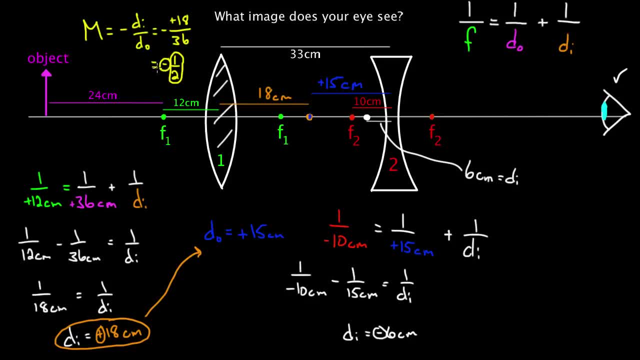 And it's going to be negative in magnification. That means it's upside down. So I'm going to draw this first image. I'm going to do it in orange, Because that's what I labeled the image distance. It's going to be upside down and half as big as the object. 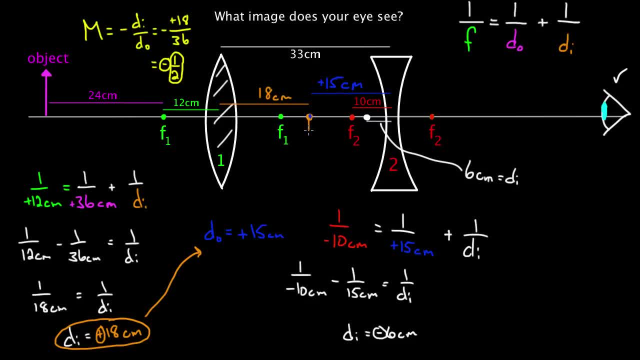 So if the object was that big, My image is going to be upside down And about half as big. So this was my image one. I'll label it image one. That's what I'm treating as my second object. So So, that's image one. 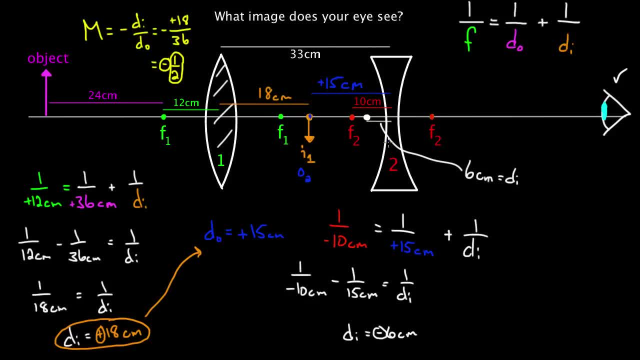 That's object two, Essentially, Because that's what this second lens is going to think- is the object. What magnification does it provide? Well, let's do that. one Magnification equals negative di Over. do So negative of My image distance. 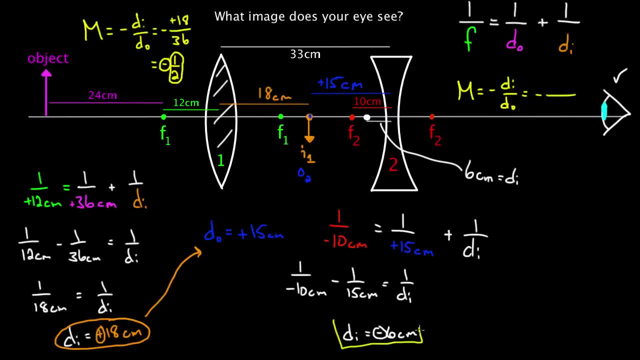 For this second lens was It was negative six. Remember, right here, That's what we solved: Negative units because they cancel. And my object distance for this second lens Was fifteen centimeters. That's what this was. right here, The distance from the lens. 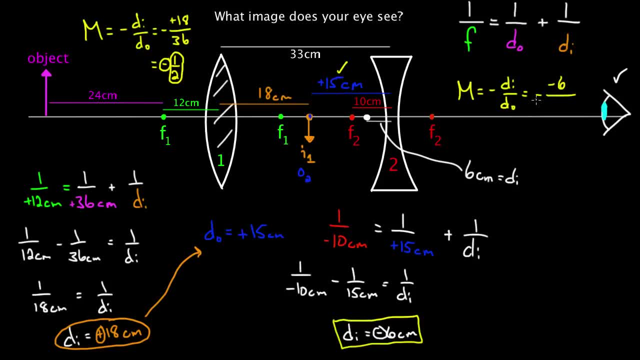 To where it's object. Quote on quote. object was, And that was fifteen, Positive fifteen. And what do I get? If you take negative of negative six over fifteen, You end up getting positive Two fifths. So this is the second magnification. 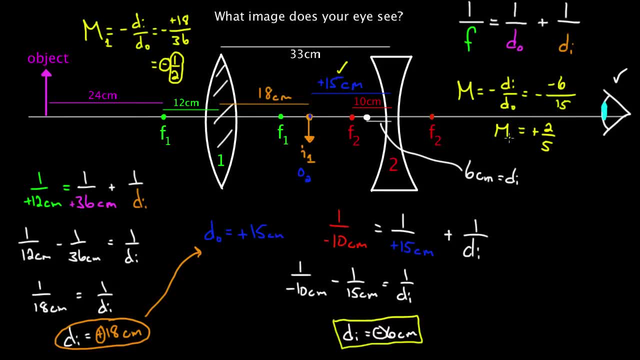 The magnification of the first lens Was negative one half. Magnification of the second lens Was positive: two fifths. That means at this point- over here I'll make it white, Because that's where I labeled this image distance- I'm going to get an image that's two fifths. 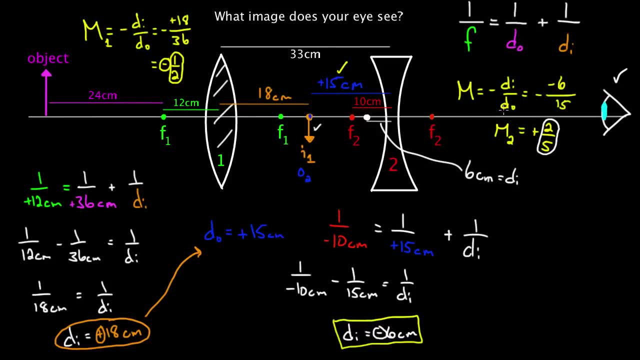 As big as what As the first image. So now this is a magnification of The image, Because that's what this second lens is doing. So I don't look back at my object over here. I'm done with this guy for now. 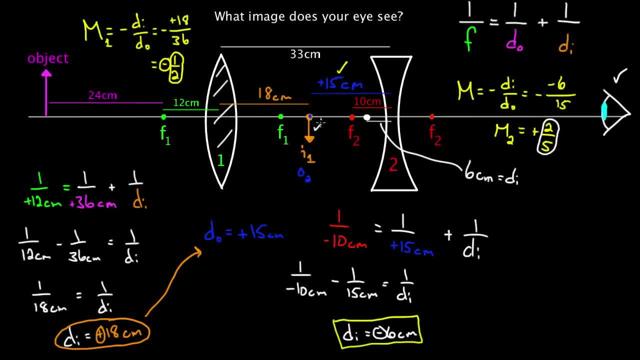 Now I'm just looking at what this second lens Is doing. So two fifths as big as this object, And positive means right side up, But in this case This really just means not inverted. So this started off Our object for this second lens. 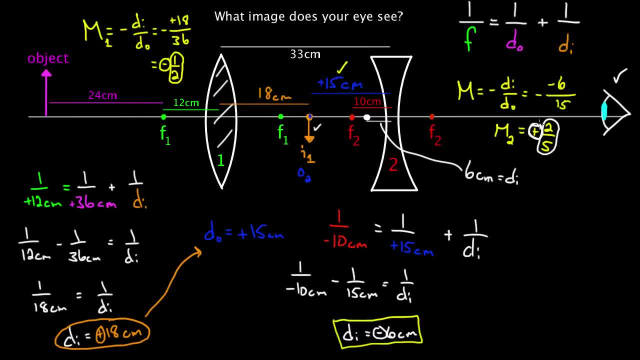 Started off upside down. This positive means that you maintain the direction, You don't invert it. So I leave this thing upside down. That's what it means. I leave it upside down. If it would have started right side up, I would have left it right side up. 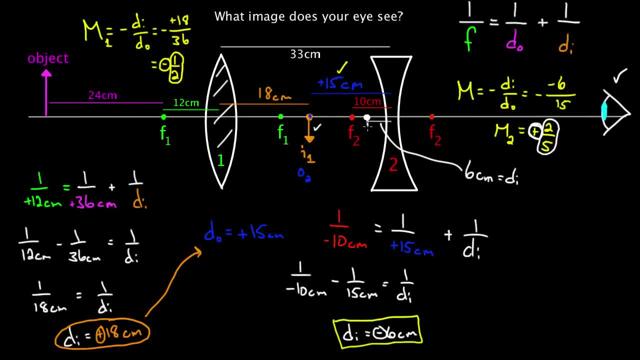 So a little under one half, And so I'm going to draw this About like that. That's where my image would be Right there. That's what I would see. I would see a very little image. That's upside down. 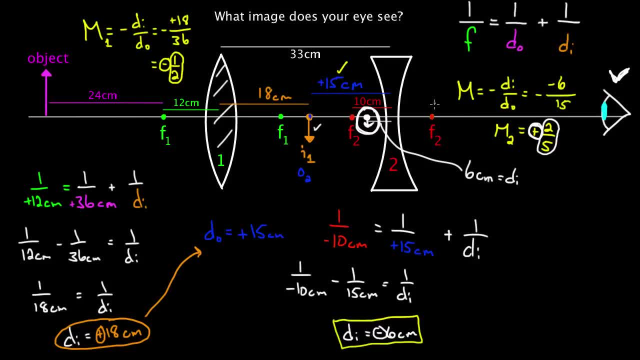 And it would be right around there, And so that's an example of where you can do A two lens system. You treat each lens separately And you use these formulas accordingly. The last thing I'll say is, If you wanted to know, 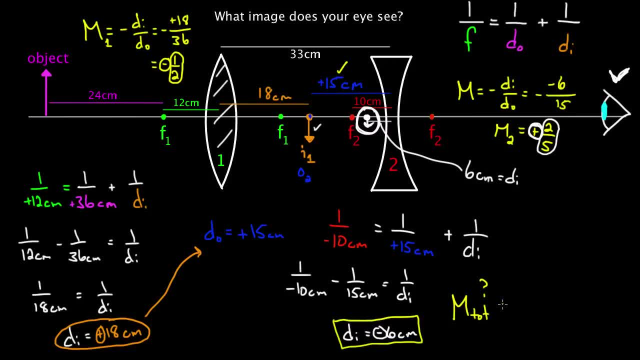 Is there some way to figure out The total magnification, Some slick way of doing it? Yeah, and it's really easy, it turns out. You can just take your total magnification. If all I wanted to know was If I had this object. 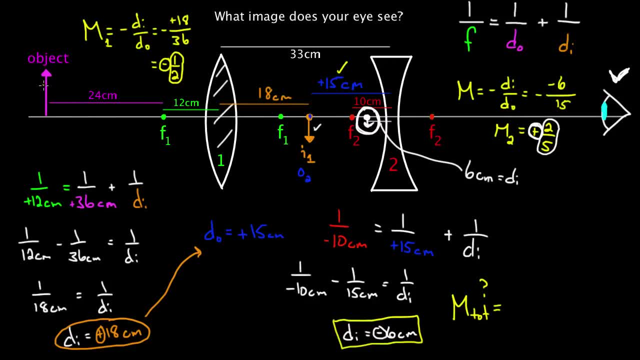 What my total magnification was going to be. What could I multiply this object's height by? In other words, What factor could I multiply it by To get the both orientation and height Of this final image? Well, you just take the magnification of the first lens. 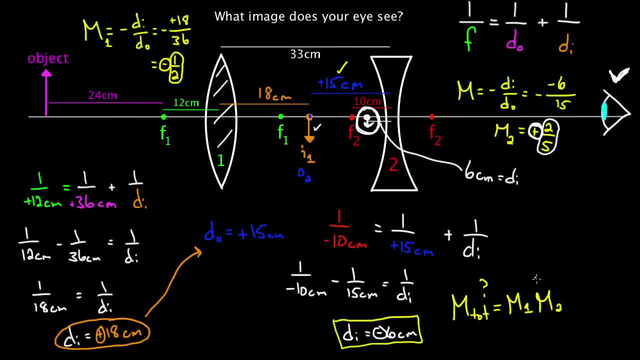 Times the magnification of the second lens. So I just multiply them all. That would give me the factor, That's the overall magnification, That I could multiply this object's height by To get the height of the final image And the orientation of it.